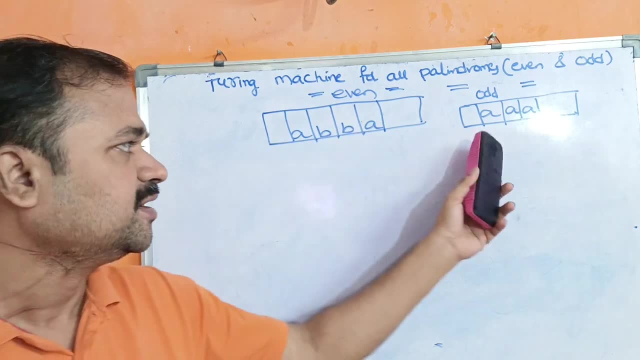 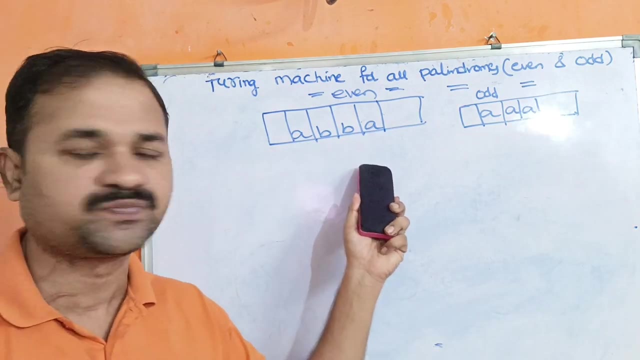 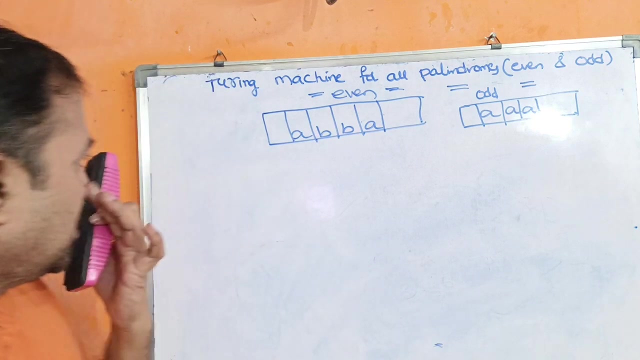 So the reverse of ABBA is ABBA only. Let the string is AAA, So the reverse of AAA is AAA only. So this is even length palindrome, whereas this is odd length palindrome. So our Turing machine has to accept both the strings. Let us design first for even palindrome, Then. 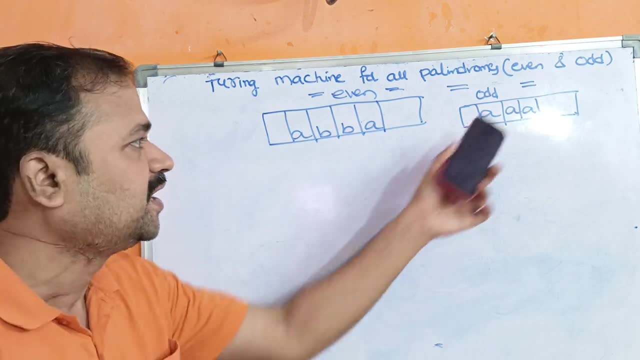 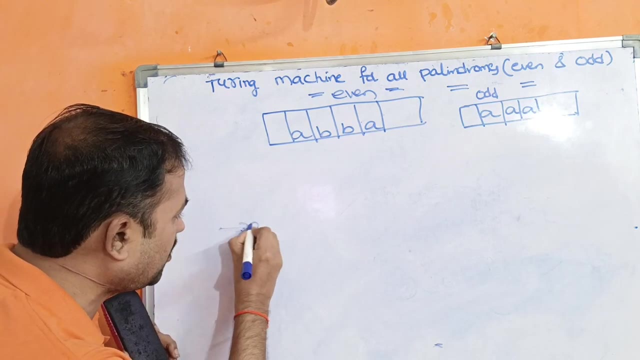 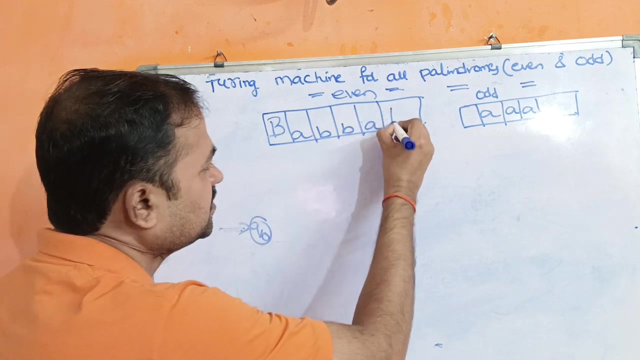 we have to make some changes in order to provide odd palindrome also. Let the starting state is CUNA. Let the starting state is CUNA CUNA. Here, before the string, we can add a number of blank symbols. After the string, we can have any number of blank symbols. So 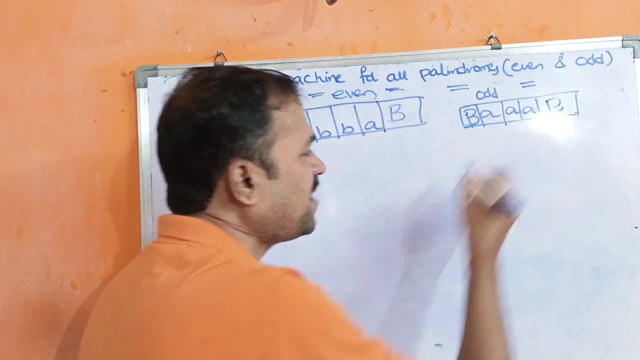 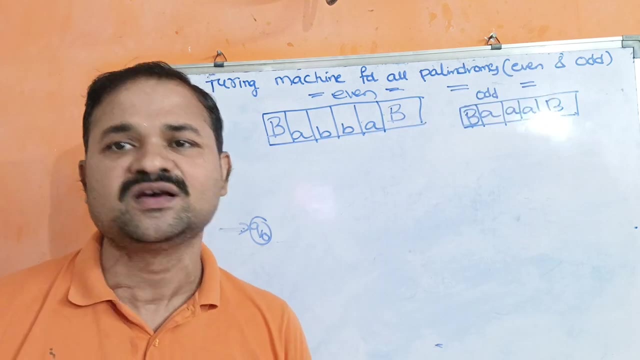 here also: before the string, any number of blank symbols. After the string, we can have any number of blank symbols, So not only these strings. we can take any type of strings According to the choice. there is no problem. So for all the strings this Turing machine can accept. 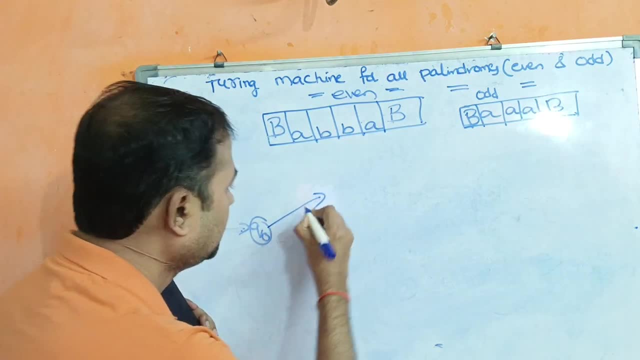 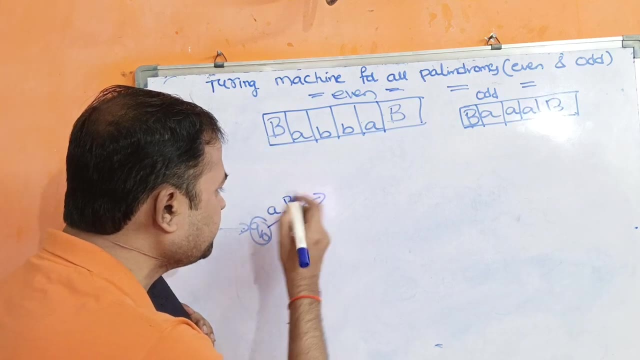 all those things, So CUNA. If we read A and CUNA then change A to CUNA, So CUNA is CUNA. Then replace A by blank symbol and move the head towards the right till we get the blank. 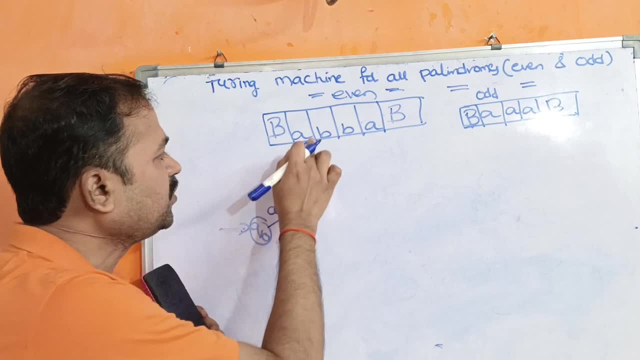 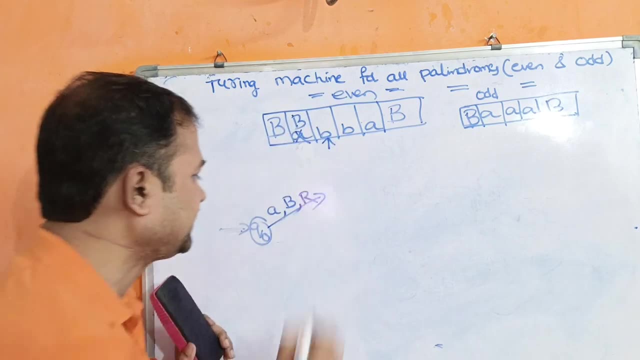 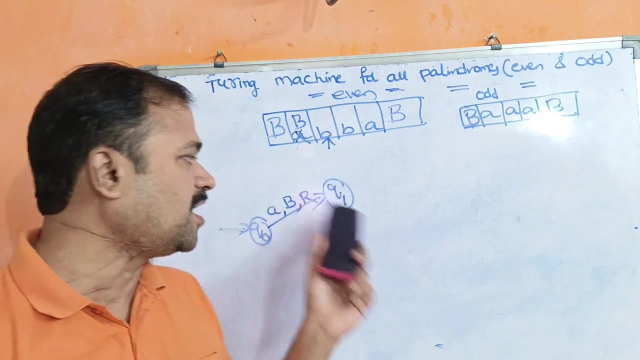 symbol. So initially we are at A. So if we read A, then what we have to do on CUNA, Then replace it by blank symbol and move one position to the right. Next we are at Q1 state. If we read A's and B's on Q1, then don't change them and move the head towards the right till. 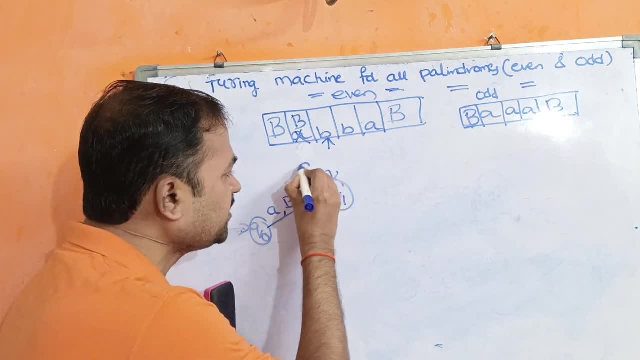 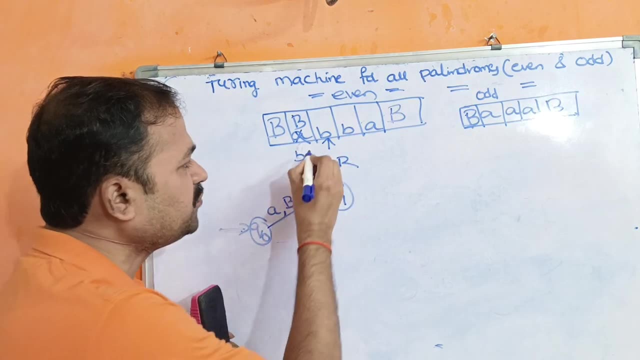 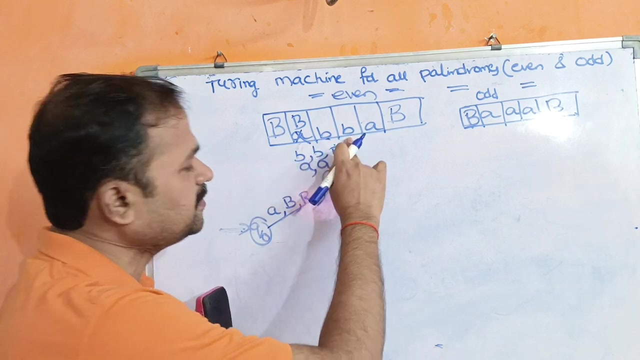 we get the blank symbol. So if we read A on Q1, don't change A, So keep it as A only, but move the head towards the right. If we read B on Q1, don't change B, but move the head towards the right. So B move one position to the right. So B move one position to the right, A move. 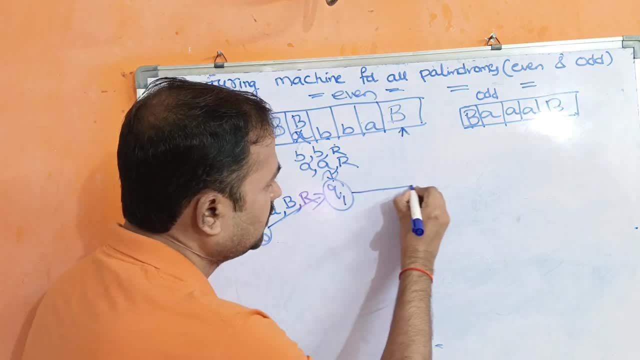 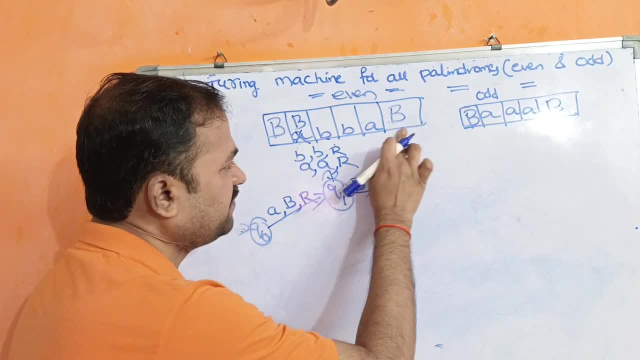 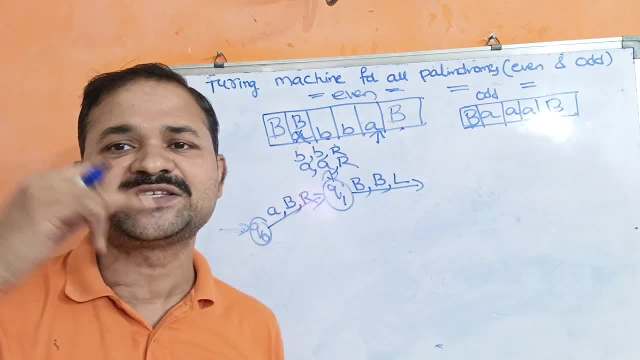 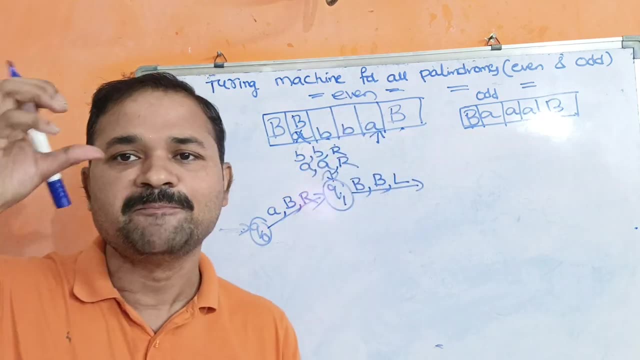 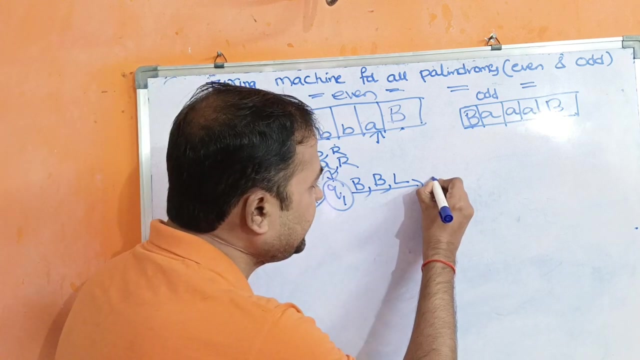 first symbol of the string is a, so that a is replaced by b, whereas the last symbol is also a. so now we have to replace this a by blank symbol and move the head towards the left till we get this blank symbol. okay, so let the state is q2 if you read blank symbol on q2. if you read blank. 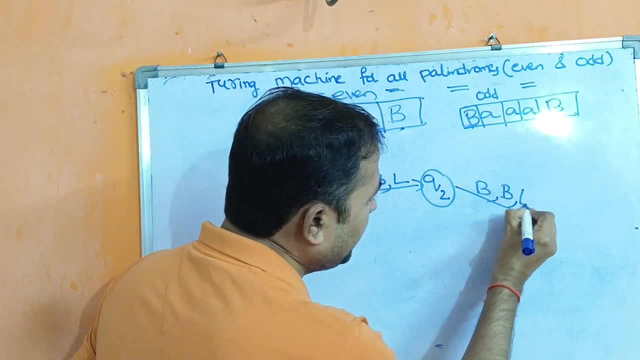 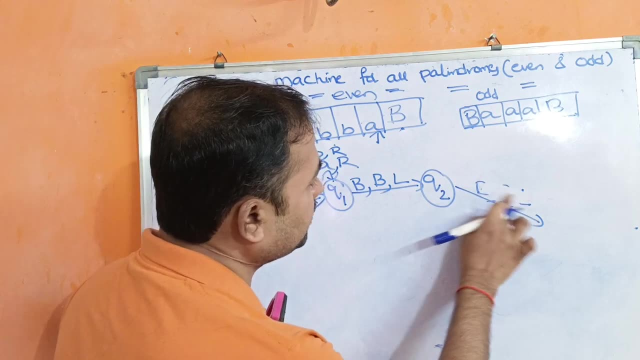 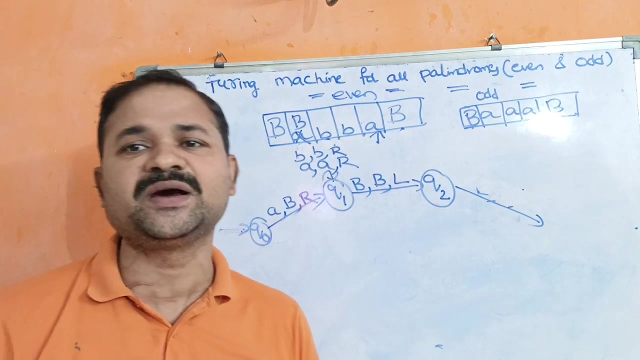 symbol on q2. don't change b, but move the head towards the left. okay, but move the head towards the left, so that that is already over. that is already over. so now we are at a. so what we have to do, we have to replace this a by blank symbol and move the head towards the left. okay, why? because 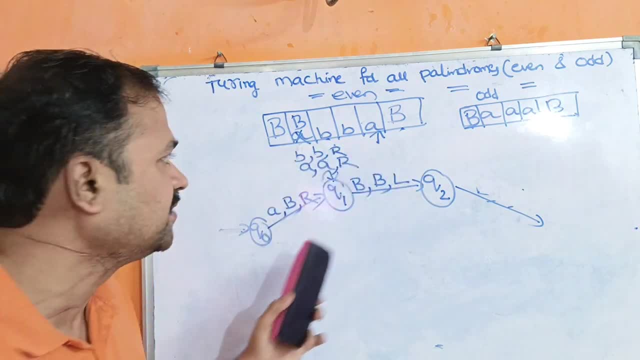 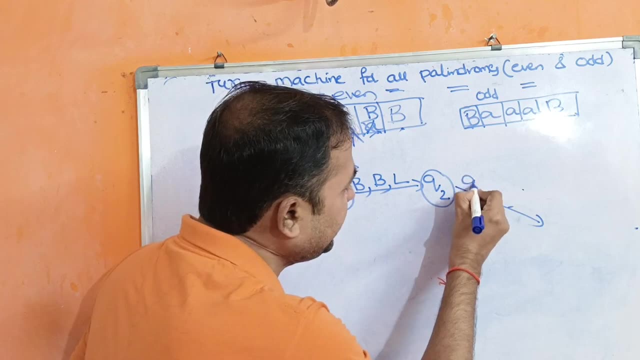 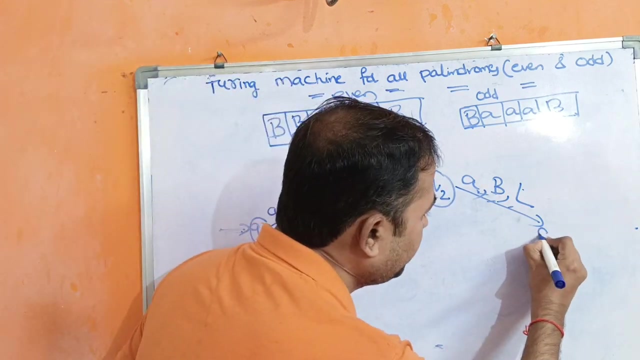 this a is for the corresponding first a. okay, so replace this a by blank symbol and move the head one position to the left. okay, so if you read a, then replace the a by blank symbol and move the head one position to the left. so now we are at q3. on q3, if we apply any number of a's and b's, 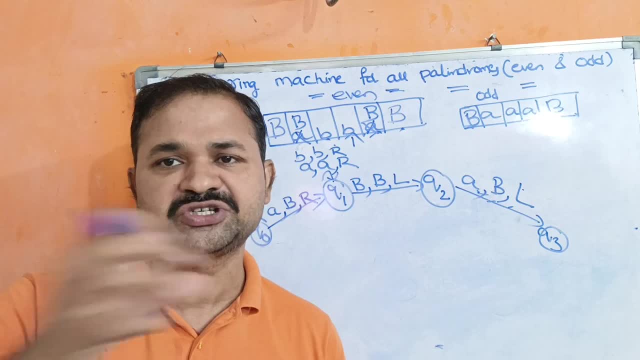 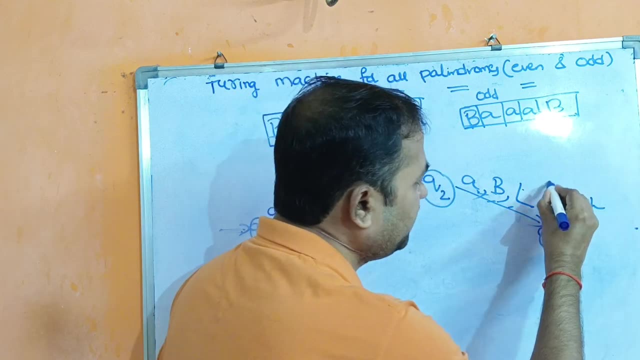 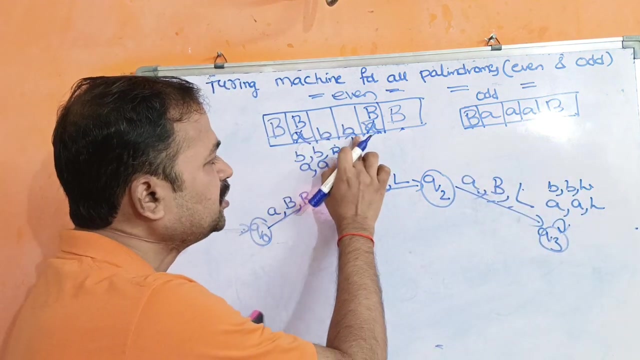 then don't change them, but move the head one position to the left. so on q3, if we apply any number of a's, don't change them, but move the head one position to the left. if you apply b, don't change b, but move the head one position to the left. here we have b. don't change b, but move one. 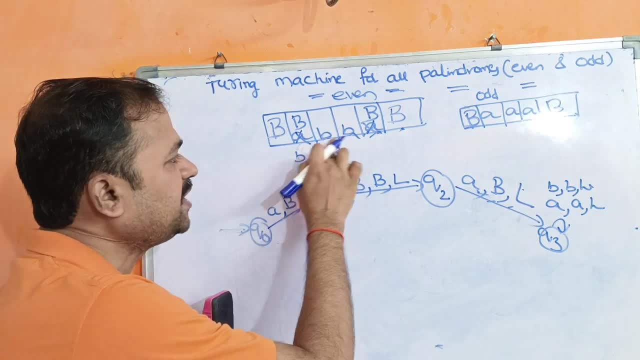 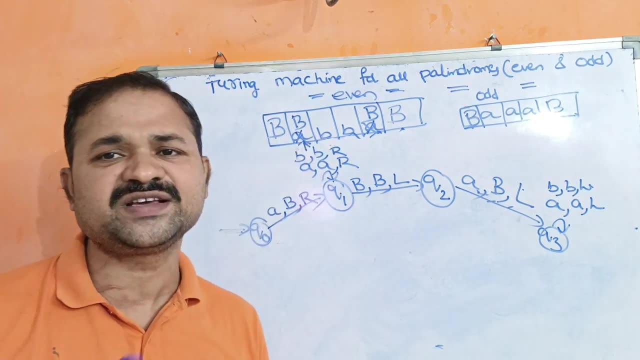 position to the left. b. don't change b, but move the head one position to the left. so next we need the black symbol. next we got the black symbol. so if you need the black symbol, then it specifies that one symbol is over. so next we have to search for the next symbol. so we need to go to the starting. 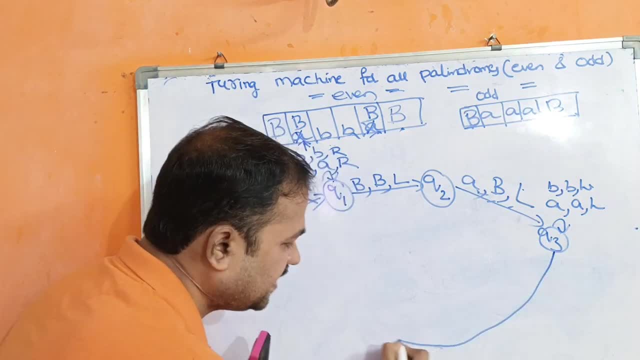 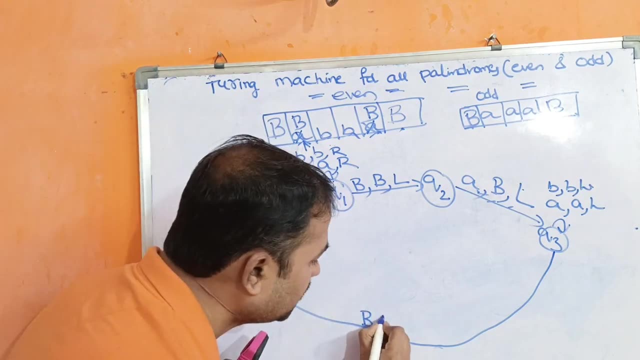 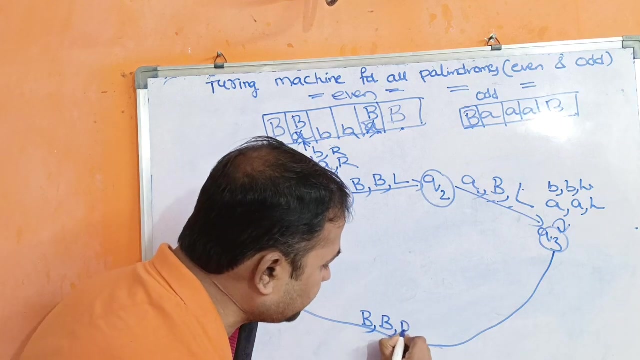 state: okay, so here we can write a transition like this. we can write a transition like this: so if you need blank symbol on the q3, don't change the blank symbol, don't change the blank symbol, but move the head one position to the right. so don't change the blank symbol and move the head. 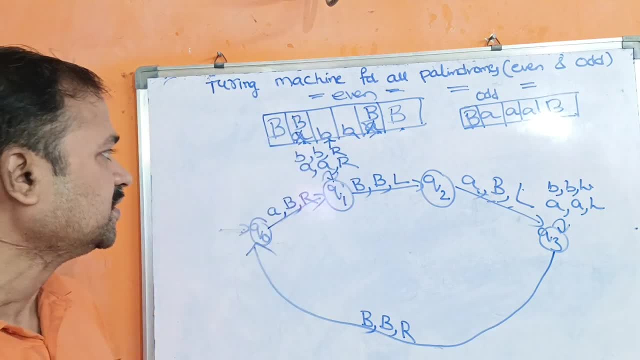 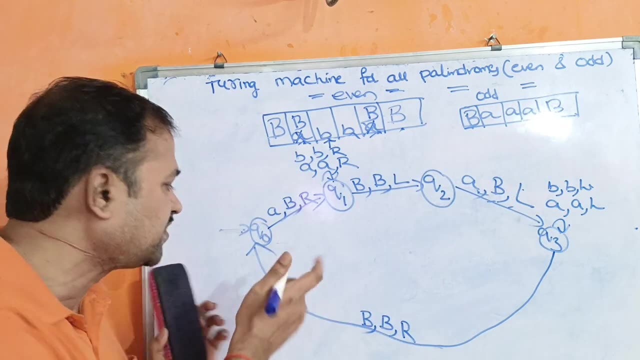 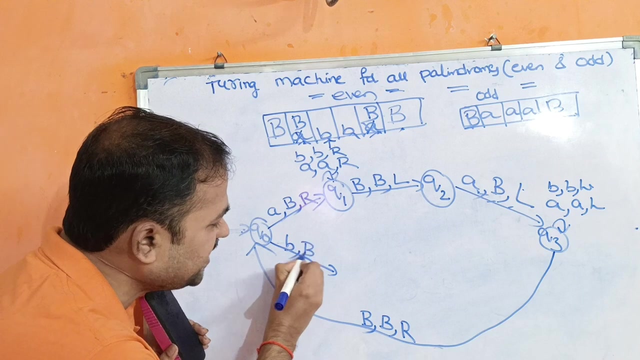 one position. so now we are here, this b, okay b. so here for a. already the path is over, all the transitions are written. now we have to search for the b. so if you read, now we have to write for the b. so if you read b on q0 state, then replace b by the blank symbol and move the head. 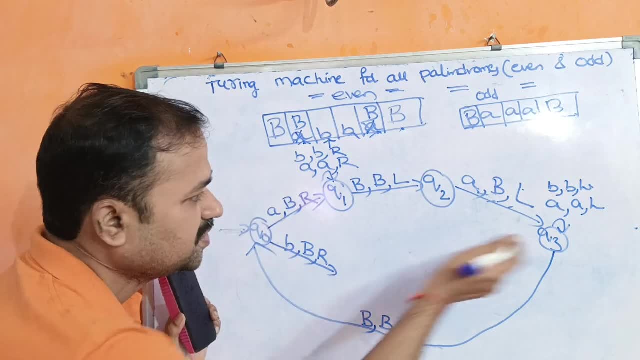 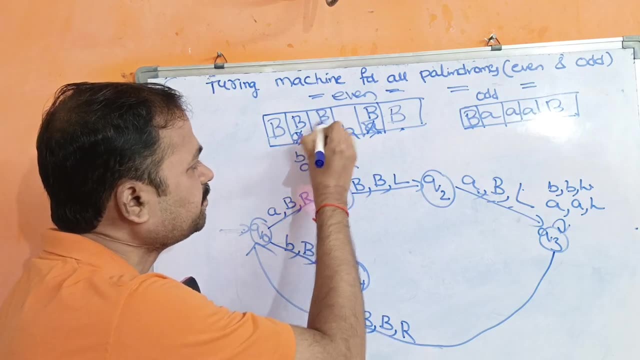 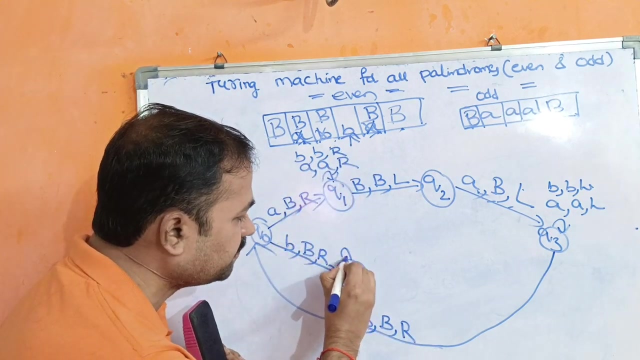 one position to the right. so this is just like this transition only. so q3 is over. let the next transition is let. the next state is q4. so replace this b by blank symbol and move the head one position to the right. okay, next on q4. q4 and q1 are similar, only. 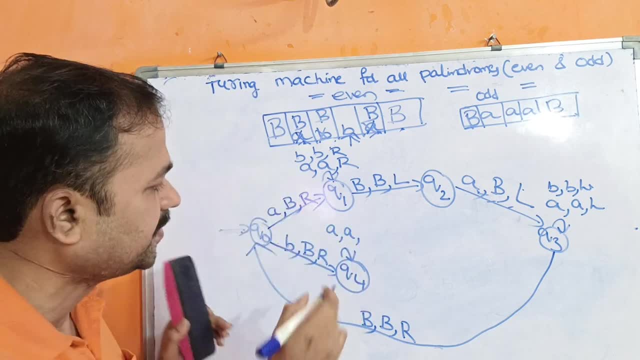 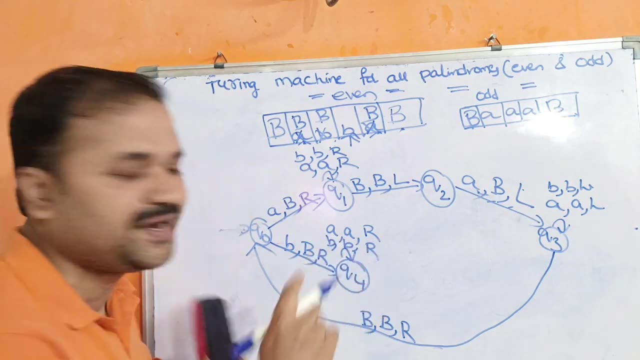 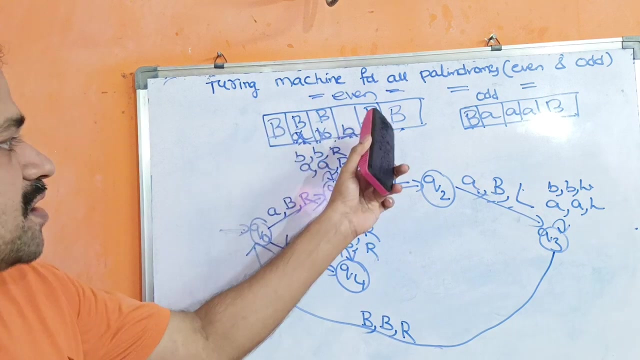 so if you read any number of years on q4, then don't change here, but move the head one position to the right. if you read b, then don't change b, but move the head one position to the right. okay, so don't change b, but move the head one position to the right. so now we got the blank blank symbol. 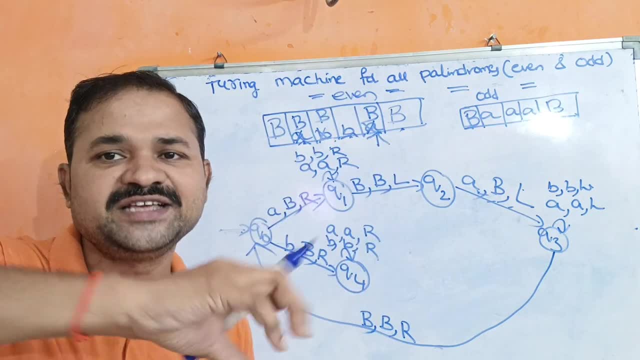 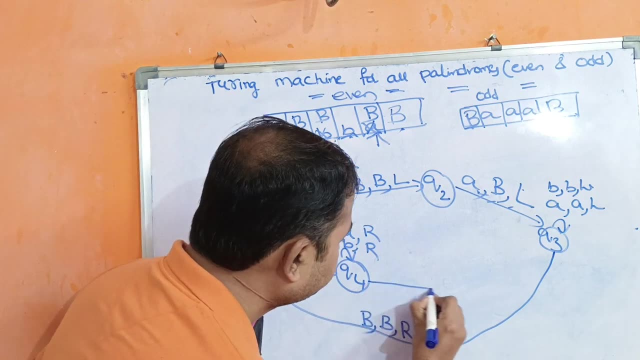 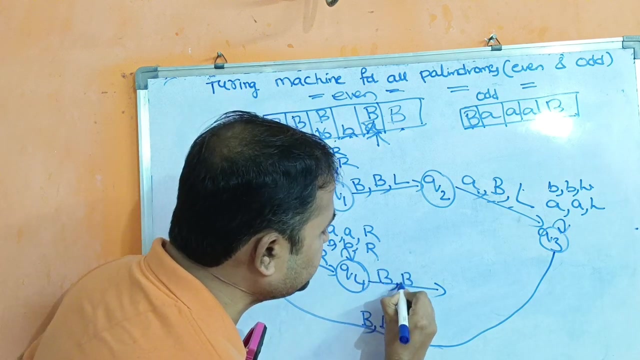 so this blank symbol specifies that we reach the end of the stream. okay, so we have to move position to the left. okay, so let we need the blank symbol. so don't change B, but move the head one position to the left. ok, move the head one position to the left. 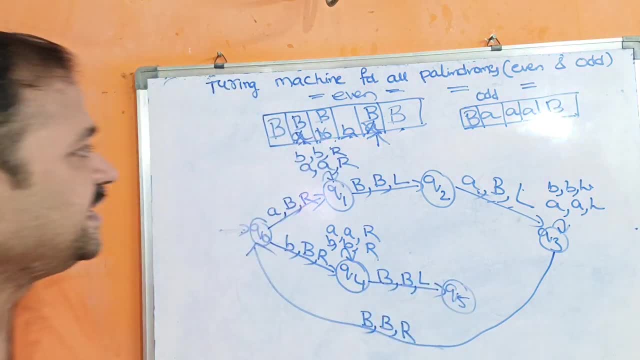 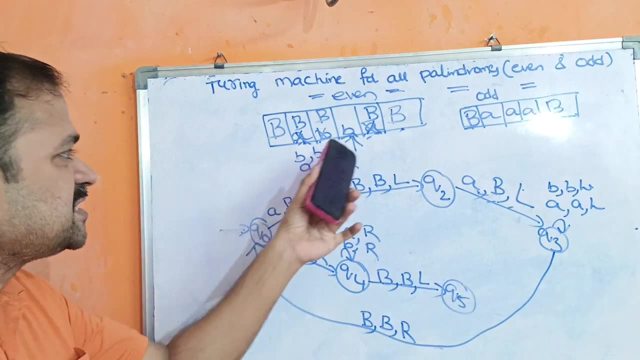 so now the state is Q5. let the state is Q5. so now we have to move one position to the left. ok, next, here we got B. so this B is for this corresponding B. ok, the second symbol from the left is 2. the second symbol from the right is 2. 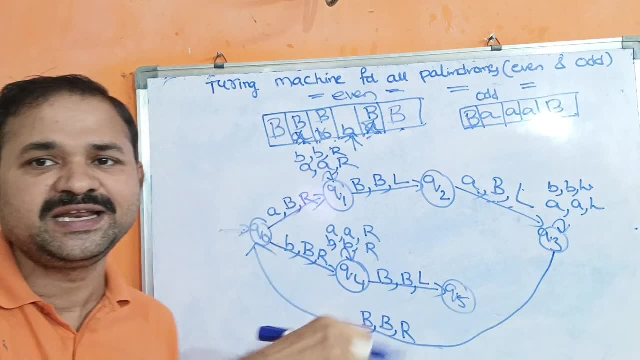 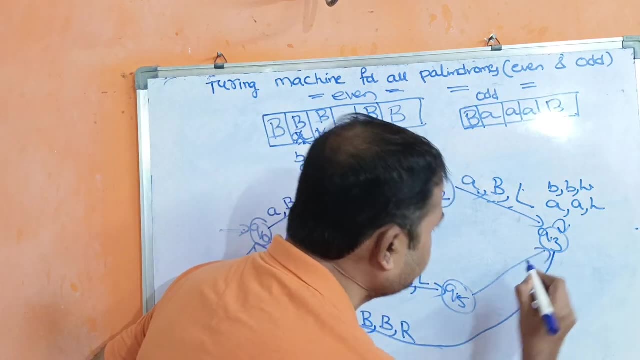 the second symbol from the left is B. that B is already replaced by blank symbol. likewise, the second symbol from the right is B, so we have to replace that B by blank symbol. so if we read B, then replace it by blank symbol and move the head one position to the left. 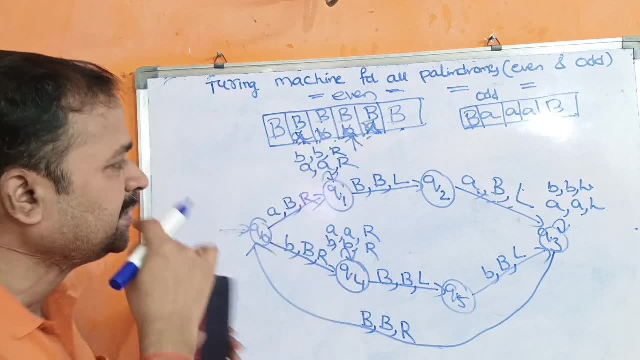 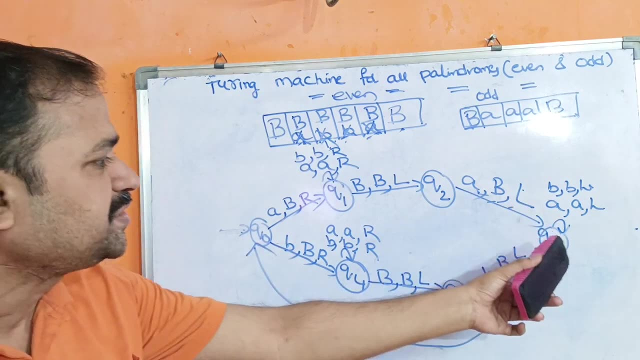 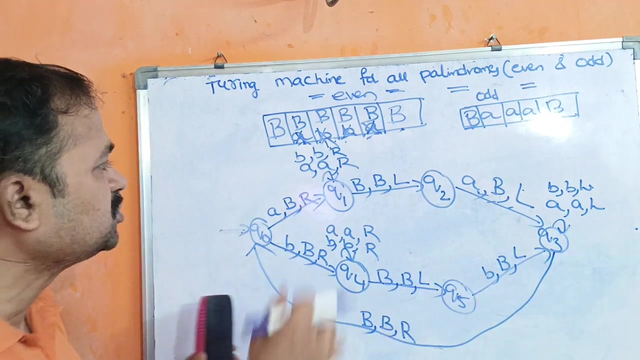 so if we read B, then replace it by blank symbol and move the head one position to the left. move the head one position to the left. so now we are at Q3, so all Q3. if we read blank symbol, then what we have to do We have to move to the unar state and move the head one position to the right. 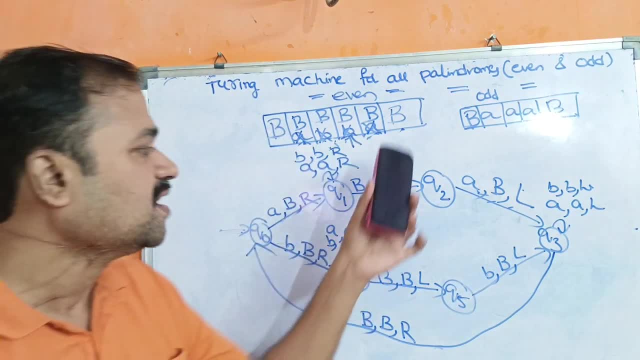 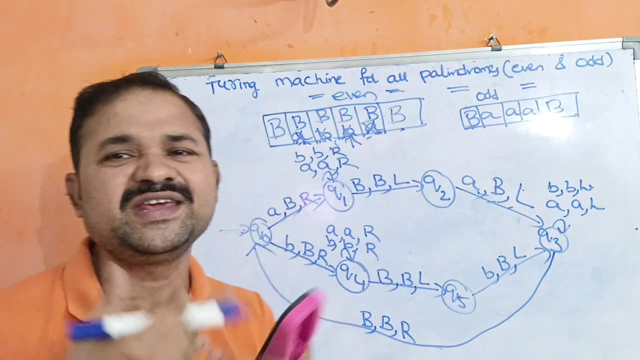 So now we are at this state. So it specifies that all the symbols are over. All the symbols are translated into the blank symbol. Why? Because we do not have any A and B. Simply, all the symbols are translated, are replaced by the blank symbol. 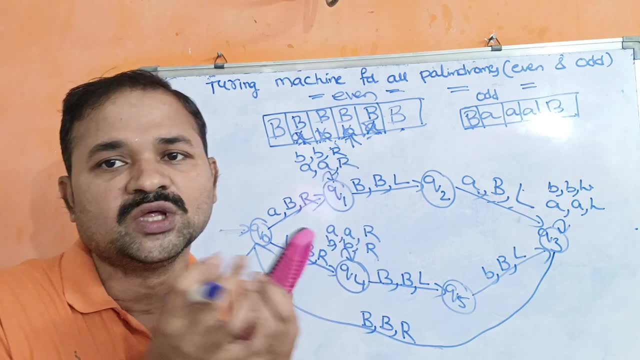 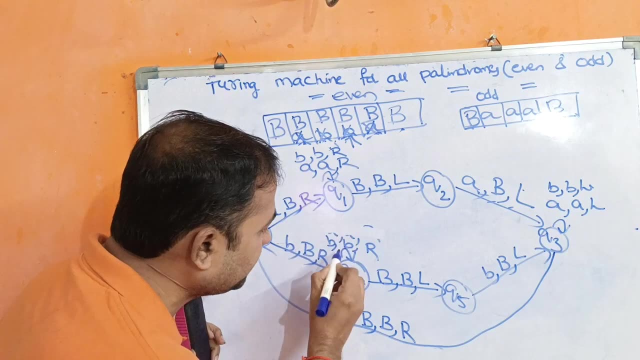 So we can say that it is a palindrome state. So now we have to go to the final state. Okay, Now we have to go to the final state. Okay, Here for space constraints. I am writing here A, So this is nothing but self-loop, self-loop transitions. 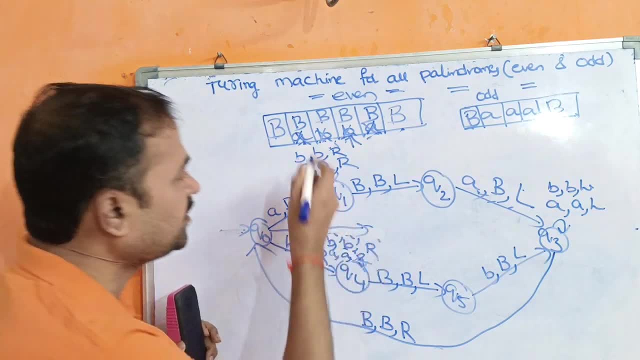 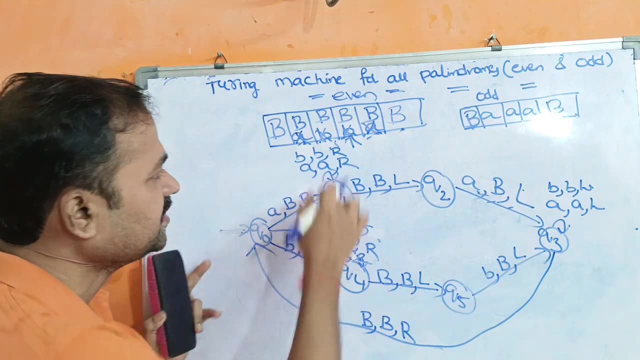 A, A right On Q0, on Q0. If we read so now we are at which state? Now we are at Q0.. Now we are at Q0.. So whenever blank symbol is reading, then what we have from Q3 to Q0. 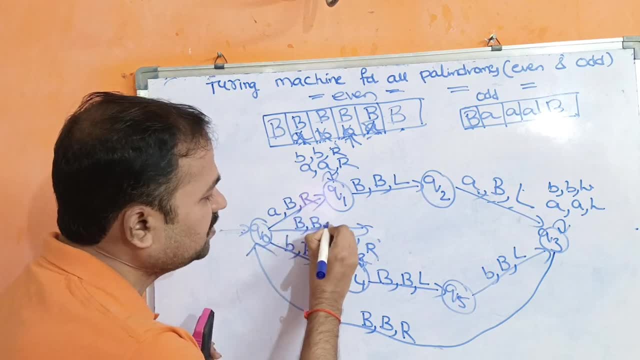 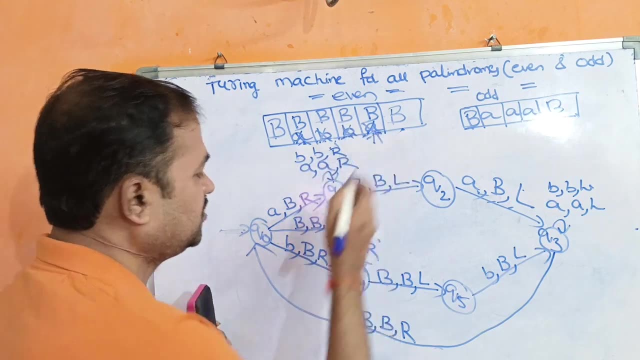 So if we read the blank symbol, then keep it here. same only. But we can move either to the left or right. It is our choice. Let us move towards the right. It is our choice. We can move towards the left also. 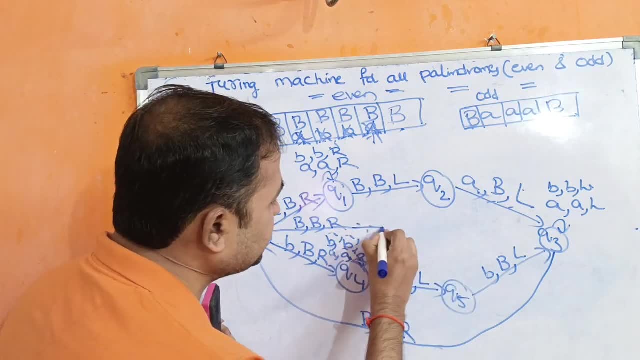 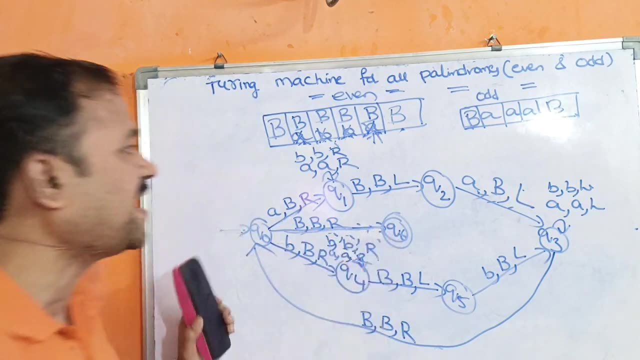 So Q5 is over. Now let the state is Q6.. Let the state is Q6.. So this is the final state. Okay, So here this path is for even palindrome, Even palindrome. So if it is an even palindrome string, that means if the palindrome string length is even. 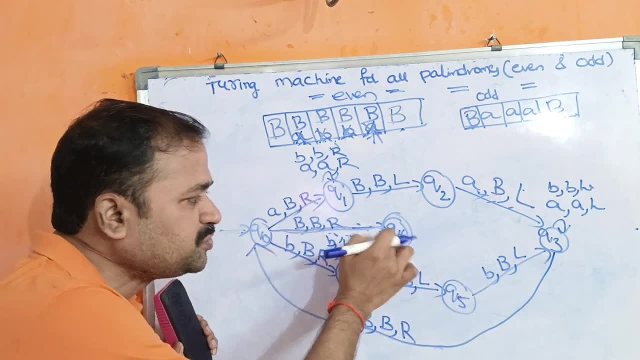 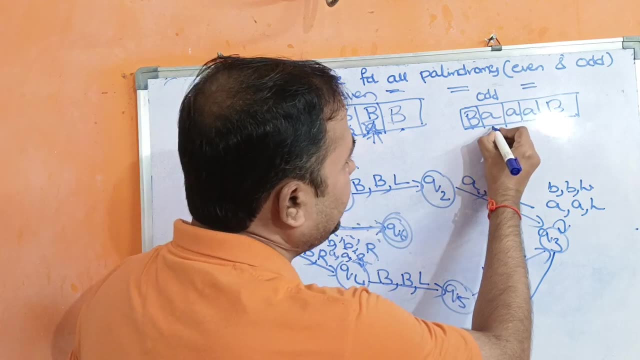 then this path reproduces the final state From Q0 to Q6, path reproduces the final state. Okay, Now let us see about the odd palindrome. So let, this is A. So what will happen first? This A will be replaced by the blank symbol. And after that we have to move the head towards the right till we get the blank symbol. And after getting the blank symbol we have to move the head one position to the left- Now this A will be replaced by the blank symbol- and move the head one position to the. 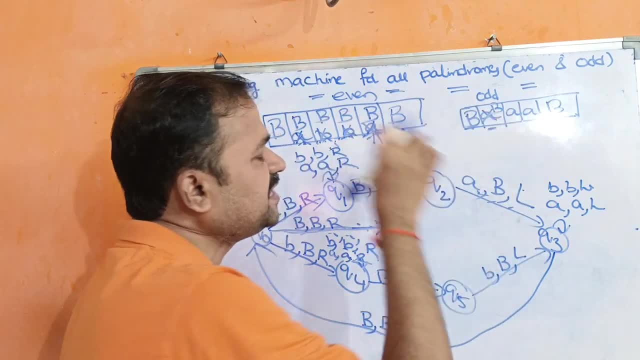 left, Move the head one position to the left And after that we have to move the head towards the left till we get the blank symbol. So whenever we get the blank symbol, we have to move the head towards the right till we. 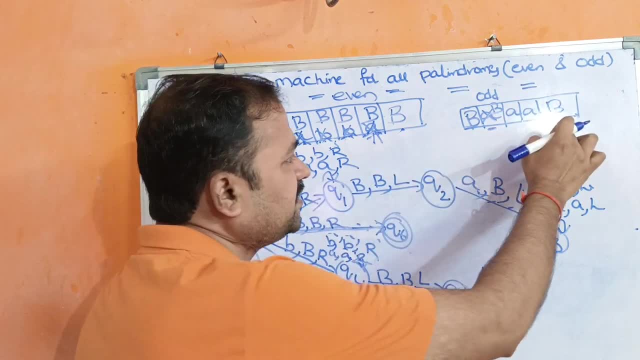 get the blank symbol. So whenever we get the blank symbol we have to move the head towards the left till we get the blank symbol. So whenever we get the blank symbol we have to move the head towards the left till we get. 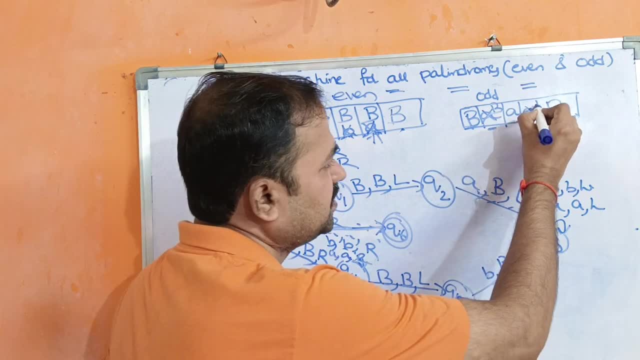 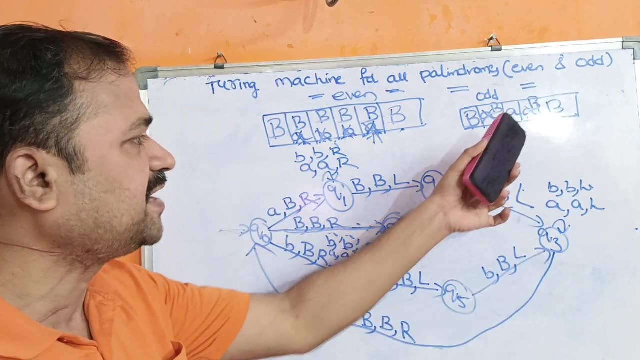 the blank symbol symbol. we have to move the head one position to the left- Now this A will be replaced by the blank symbol- and move the head one position to the left. move the head one position to the left and after that we have to move the head towards the left till we get the. 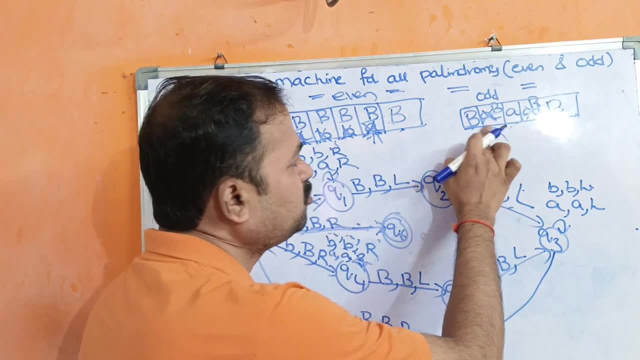 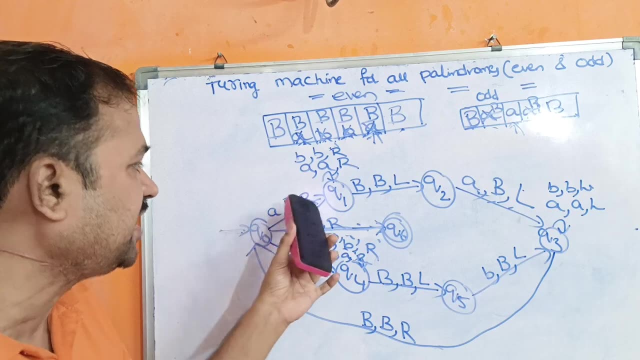 blank symbol. So whenever we got the blank symbol, then we have to simply move the head one position to the right, one position to the right, If you see this diagram. next we have A, So that A will be replaced by the blank symbol. So this A will be replaced. 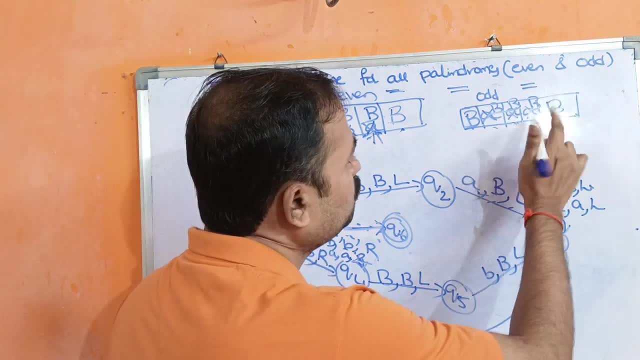 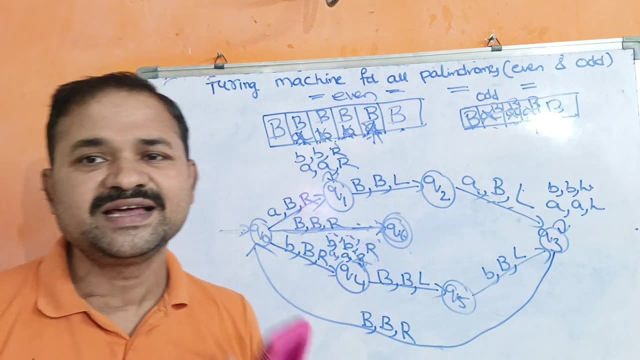 by the blank symbol and after that we have to move the head towards the right. so now we are at this position and we are at q1 state. so what will happen now? if you read blank symbol, then it specifies that there are no other symbols. all the symbols are replaced by the blank symbols. then keep it. 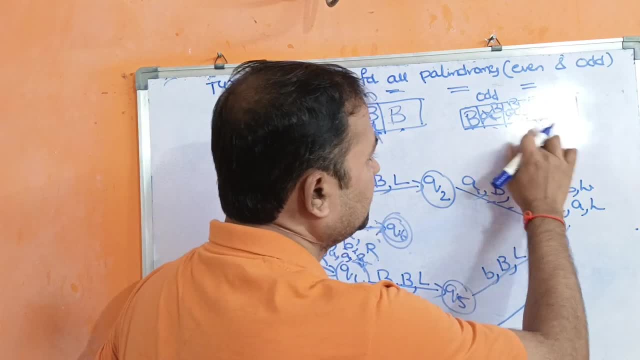 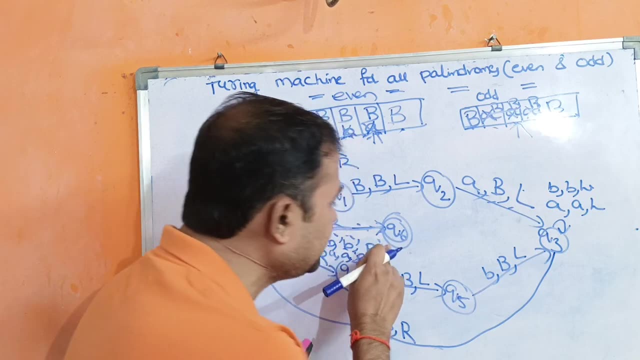 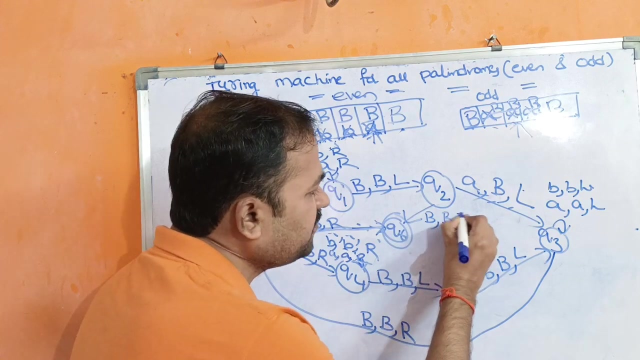 as the blank symbol only, but move the head one position to the left so we can say that this, this is also a pan-drops thing. now we have to go to the final state. so in order to go to the final state, already we have q6. so here, if you read b on q2, then don't change b, but move the head one position. 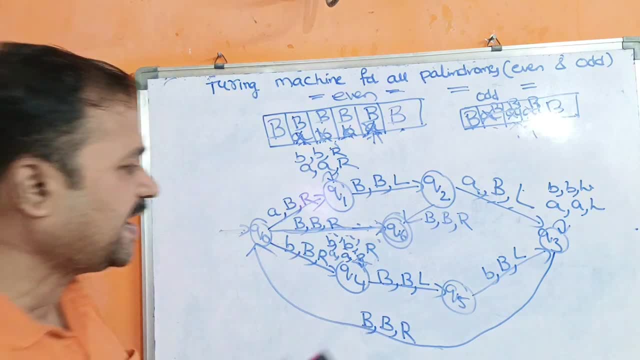 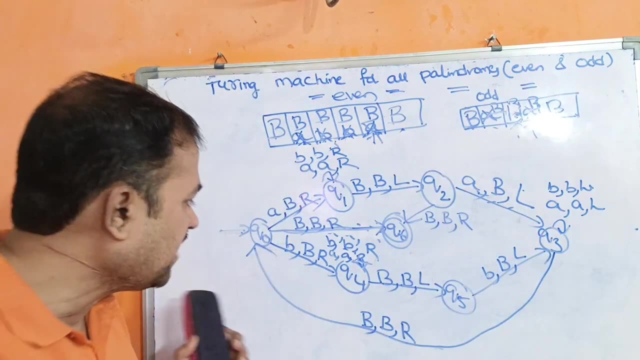 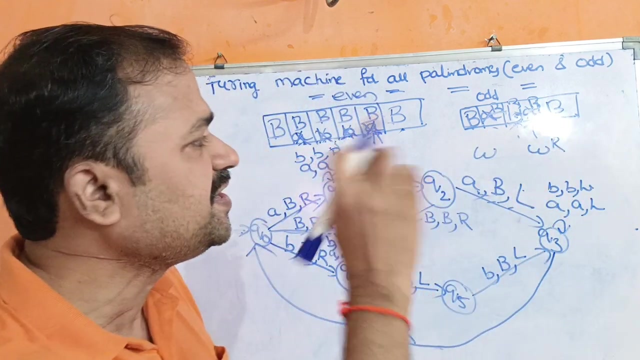 to the right. okay, so now we are at this position. okay, likewise. likewise in between aa if you have b. if you have b, then what will happen in between aa if you have b? why? because here the string is wwr in between w and w power, or we may have either a or b. here w means a. 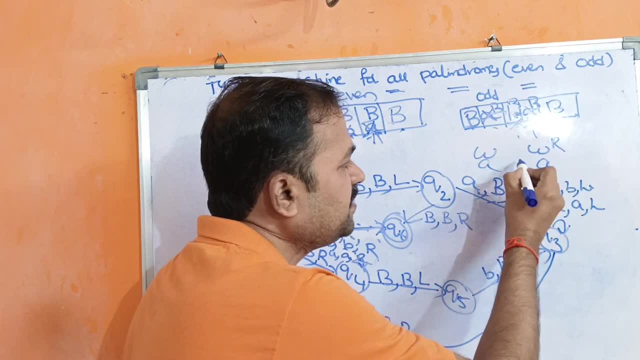 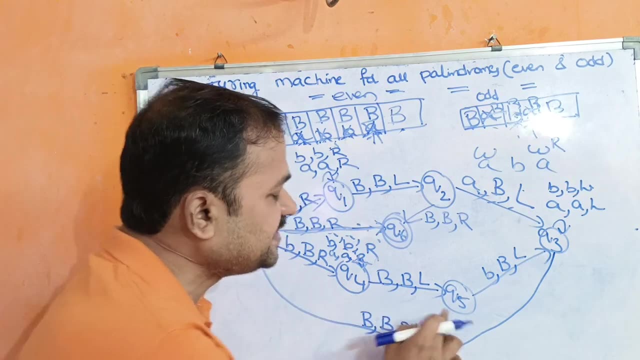 you, uh, you, you. What is the reverse of W? A only? So in between A, A we can have either A or B. Let me have B. So if we read B, then we will go in this path. Then Q5 will generate the final state. 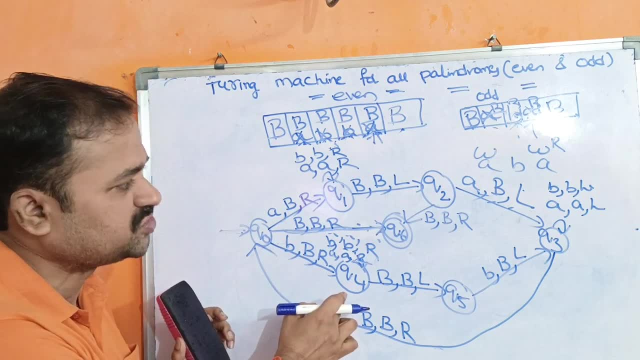 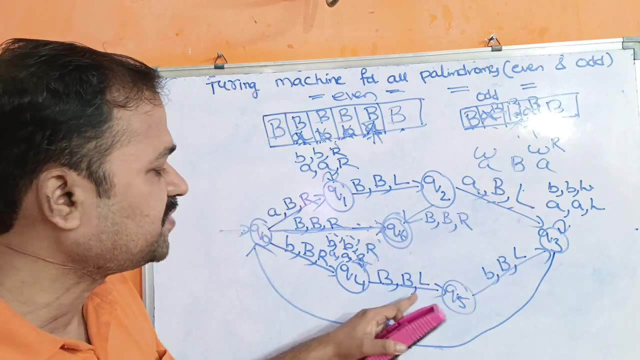 Why? Because if we read B, then what will happen? We will go to the Q4 state. We will go to the Q4 state. So this B is replaced by the blank symbol. And after that, what will happen? If we read A, we will have to. this A is replaced by B. this A is replaced by B. 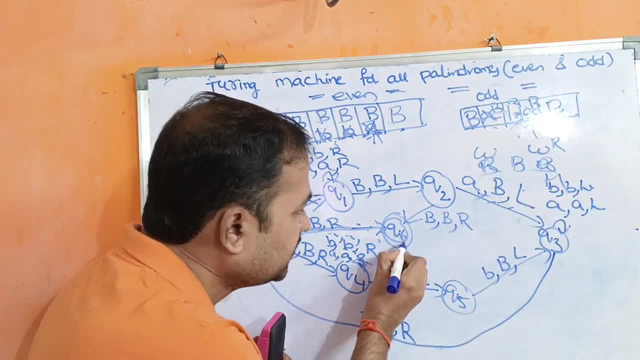 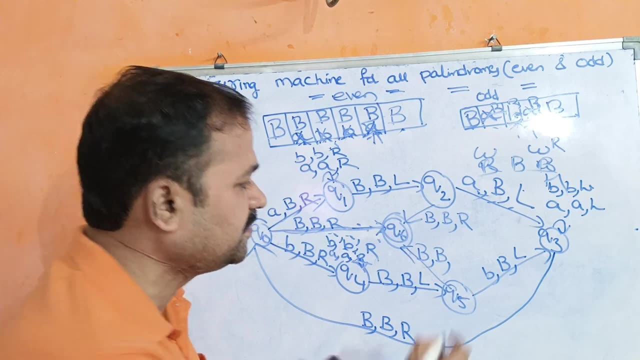 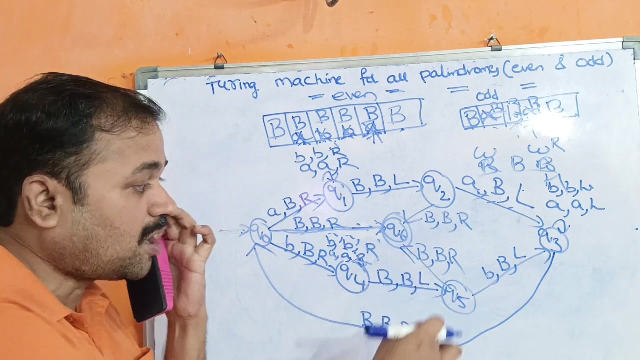 So now we are at this position And we are at Q5 state. So whenever we read blank symbol on Q5, then replace it by B only, So that means don't change B and move ahead towards the right. So here the point is this transition, this path, and this path produces all time drops.